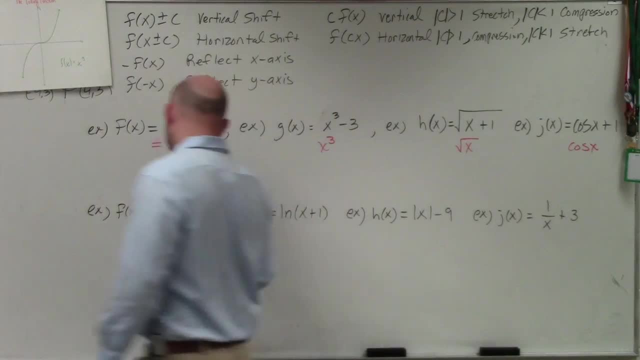 Here cosine of x is my parent function, Here 1 over x is my function, Here ln of x is my function, Here absolute value of x is my function, And here 1 over x is my function. Okay, 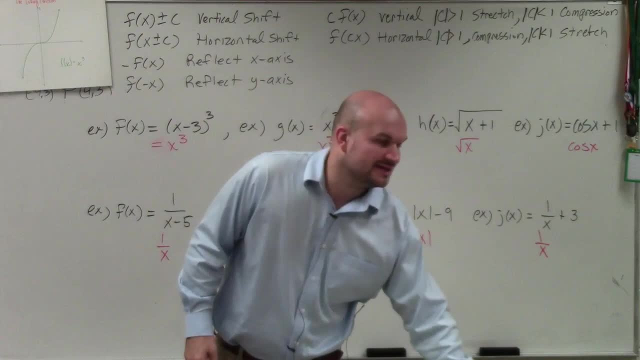 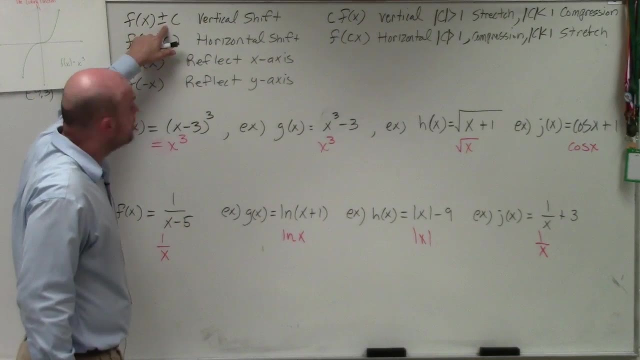 Alright now, once we've kind of identified what the function is, now what we need to do is identify: Are we applying our transformation outside the function or inside the function? You guys kind of see how there's a little difference there. So we look at the first one. 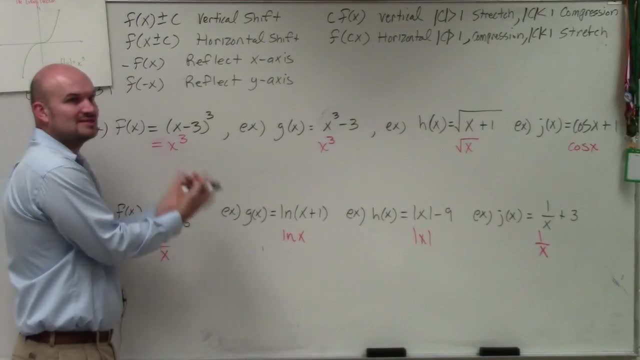 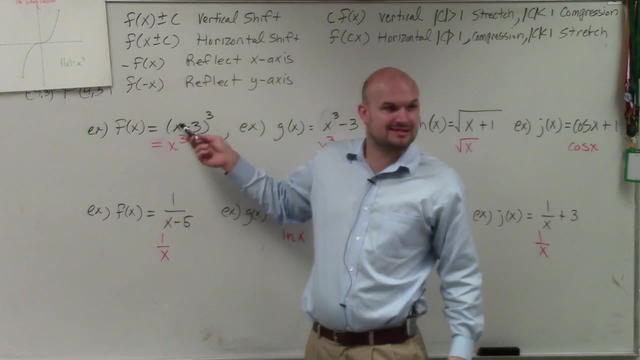 When I'm subtracting that 3,, is that inside the function or outside the function? Inside, And a good way to kind of see if it's inside the function is look to see if it's inside parentheses. Is it inside parentheses? Is it under a radical? 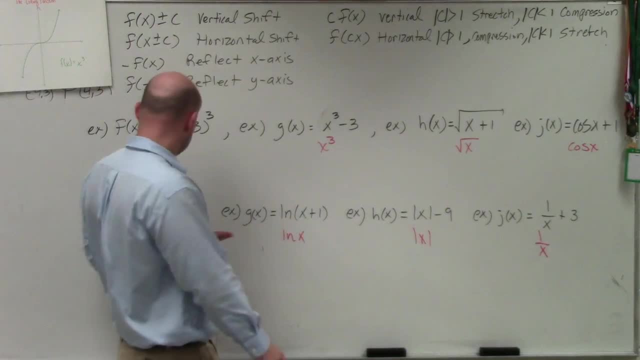 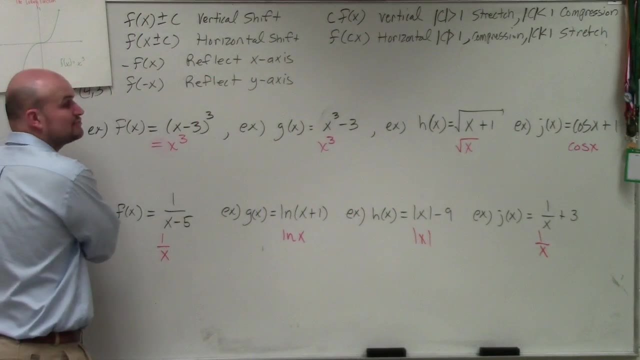 Is it in the denominator? Is it? Is it inside parentheses under a radical or in the denominator? Good ways to understand if it's inside something or not. So here you can say: I'm subtracting 3.. Now, based on that, that means it's a horizontal shift. 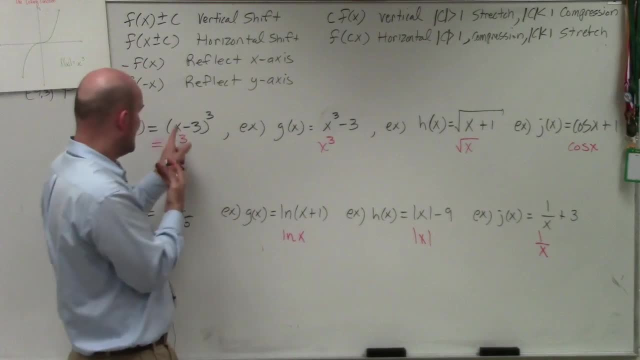 But remember, horizontal shifts were in the opposite direction, right, Because that's x minus h, So that means it's positive 3.. So that means we're going 3 units to the starts with an r, Right, Okay? 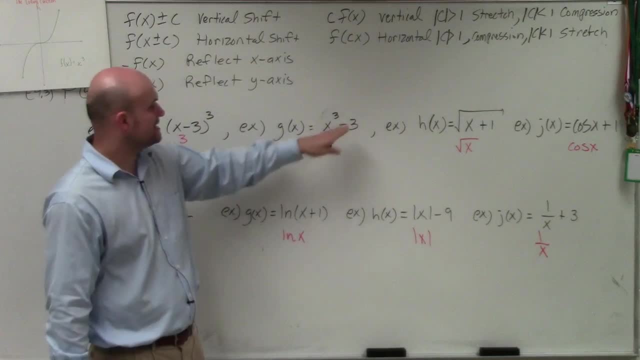 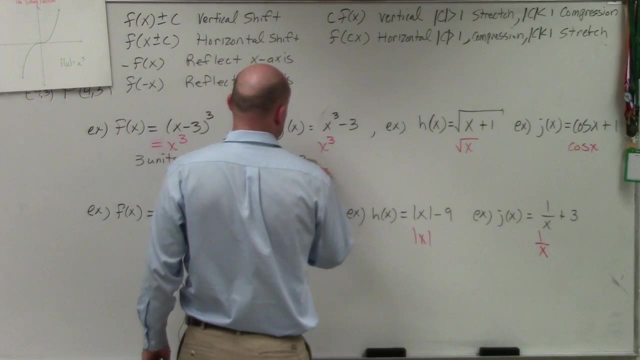 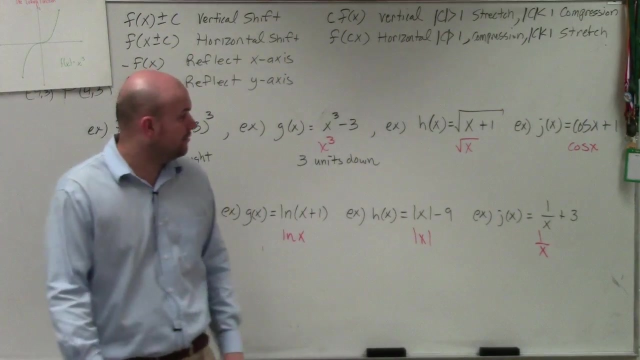 Okay, here, same function. See, I'm subtracting 3 outside the function. So now I'm shifting the graph 3 units down Here. what we have to do is determine: am I adding a 1 inside the function or outside the function? 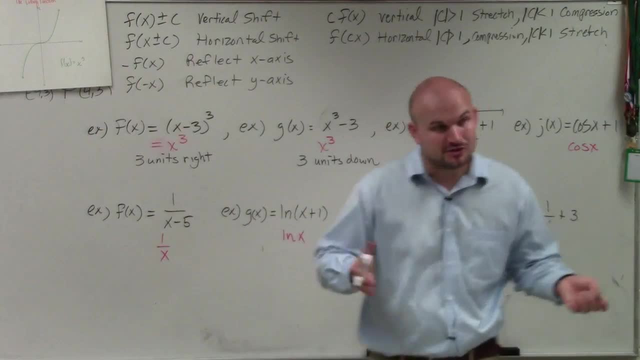 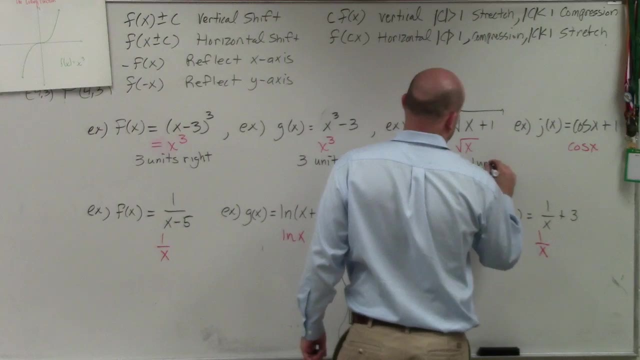 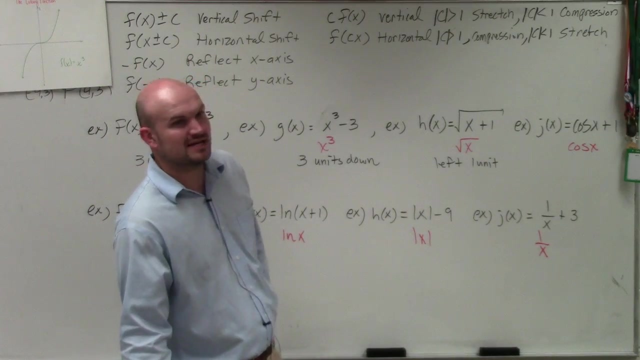 We can say Inside, Inside the function, But I'm adding, So therefore that's the same thing as going to the left. So it's left 1 unit Here. I have cosine. I need to determine am I adding a 1 inside cosine or outside of cosine? 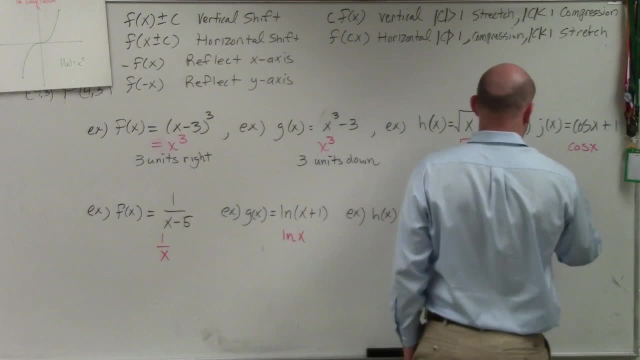 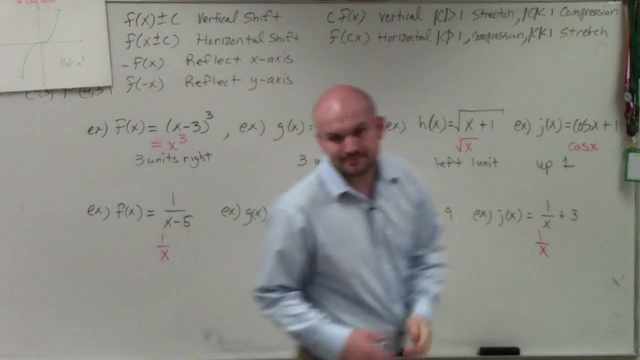 Outside, Outside. So since you're adding 1 outside, that's going to let go Up Up. Remember, outside is up down, Inside is left right. Okay, So over here I'm subtracting a 5.. 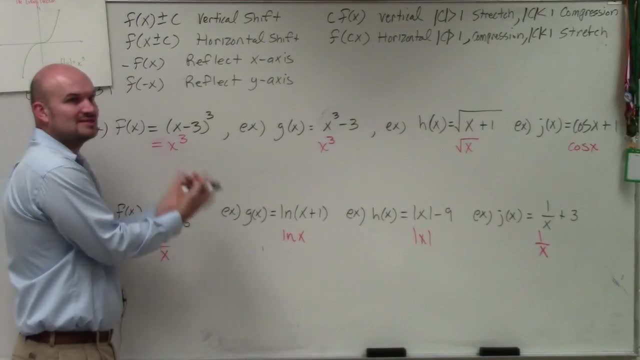 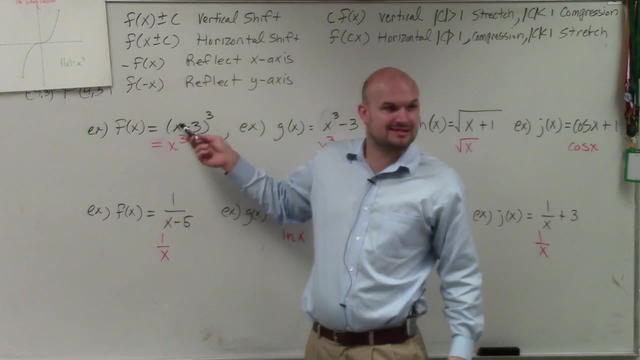 When I'm subtracting that 3,, is that inside the function or outside the function? Inside, And a good way to kind of see if it's inside the function is look to see if it's inside parentheses. Is it inside parentheses? Is it under a radical? 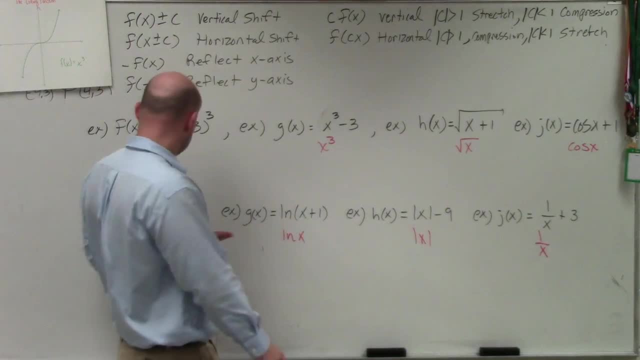 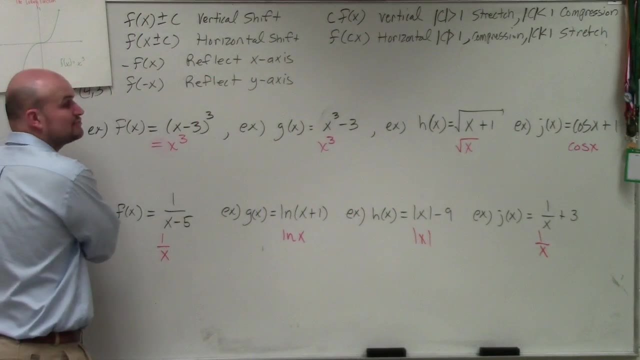 Is it in the denominator? Is it? Is it inside parentheses under a radical or in the denominator? Good ways to understand if it's inside something or not. So here you can say: I'm subtracting 3.. Now, based on that, that means it's a horizontal shift. 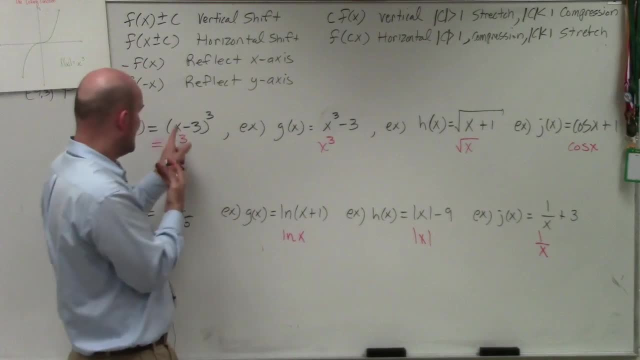 But remember, horizontal shifts were in the opposite direction, right, Because that's x minus h, So that means it's positive 3.. So that means we're going 3 units to the starts with an r, Right, Okay? 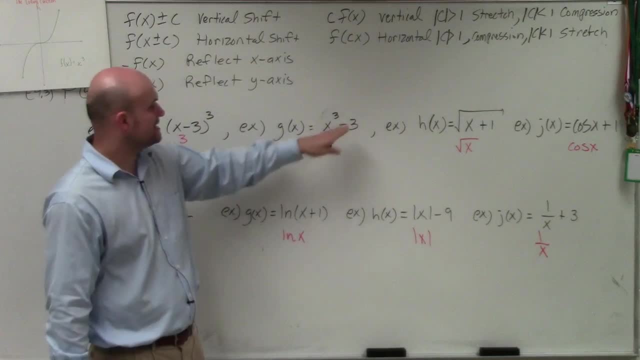 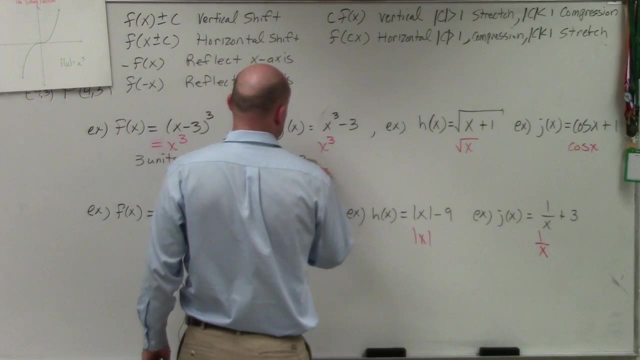 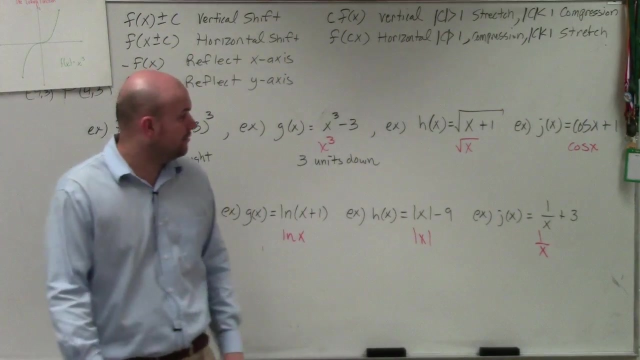 Okay, here, same function. See, I'm subtracting 3 outside the function. So now I'm shifting the graph 3 units down Here. what we have to do is determine: am I adding a 1 inside the function or outside the function? 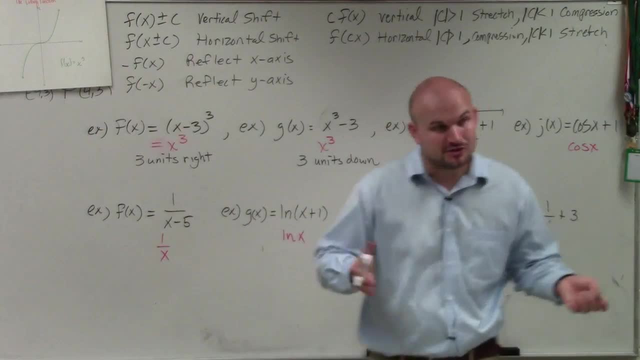 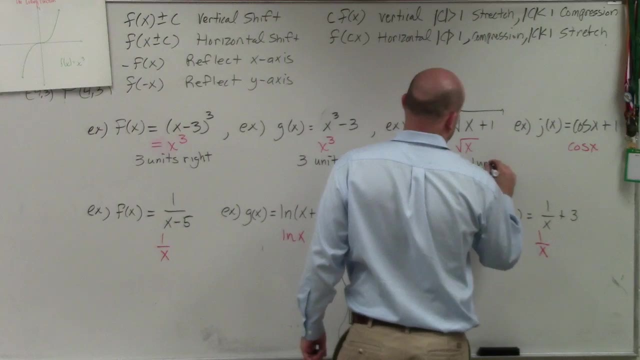 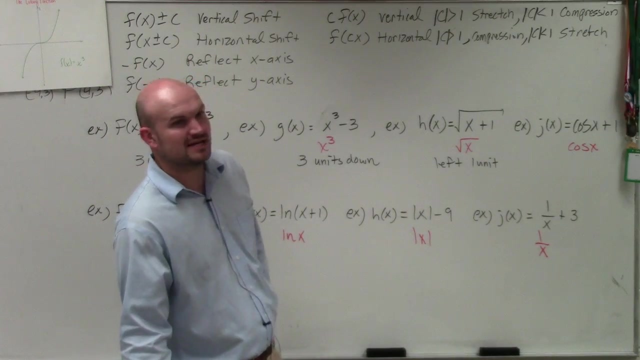 We can say Inside, Inside the function, But I'm adding, So therefore that's the same thing as going to the left. So it's left 1 unit Here. I have cosine. I need to determine am I adding a 1 inside cosine or outside of cosine? 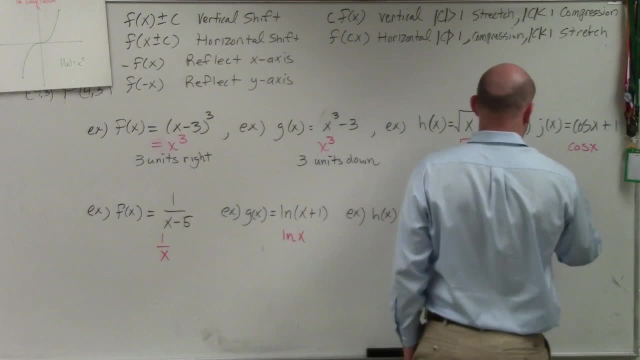 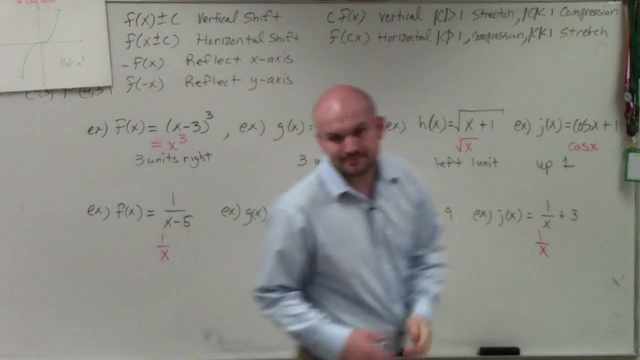 Outside, Outside. So since you're adding 1 outside, that's going to let go Up Up. Remember, outside is up down, Inside is left right. Okay, So over here I'm subtracting a 5.. 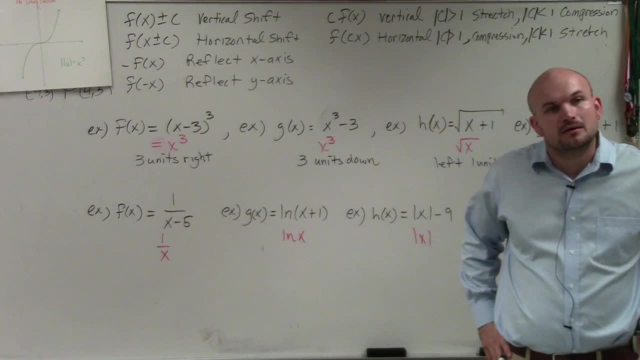 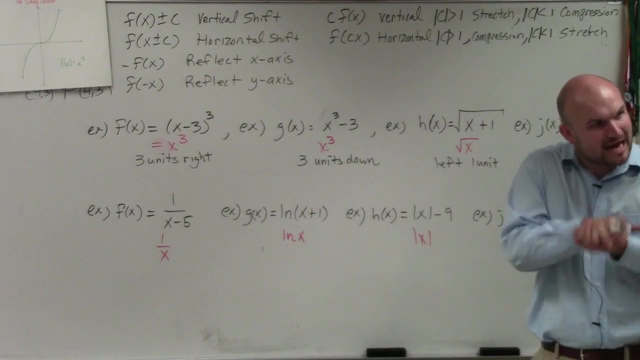 Anybody else? We got 1 for outside. Yes, Okay. So what does it mean? So if it's in the denominator, is that outside or inside the function, Inside, Inside? So if it's in the denominator, you could say it's technically inside. 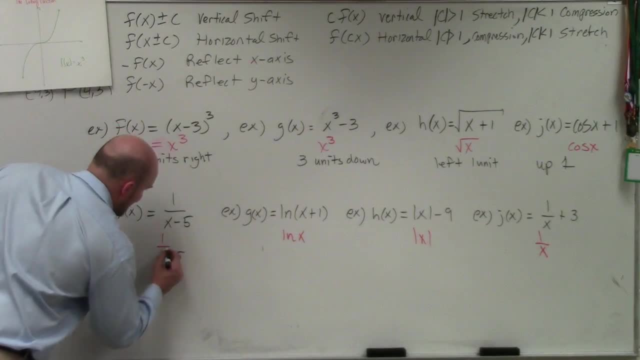 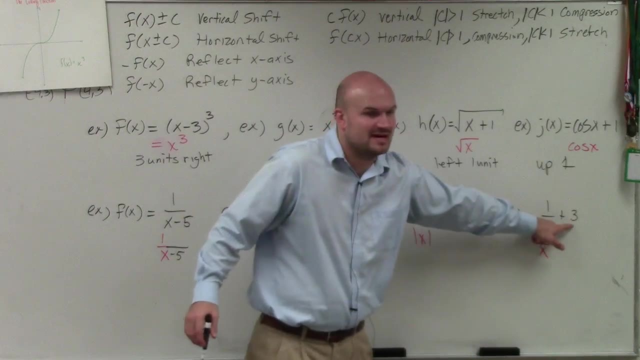 Because, think about it, Like: here's my function- I'm really subtracting a 5 inside that, like in that denominator. But when I subtract it outside the denominator, like, here's an example of outside, That's an example of inside. 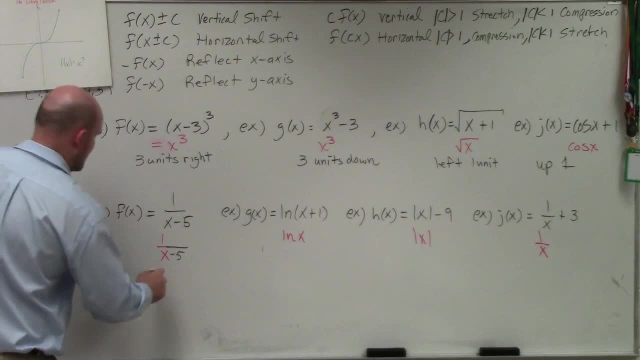 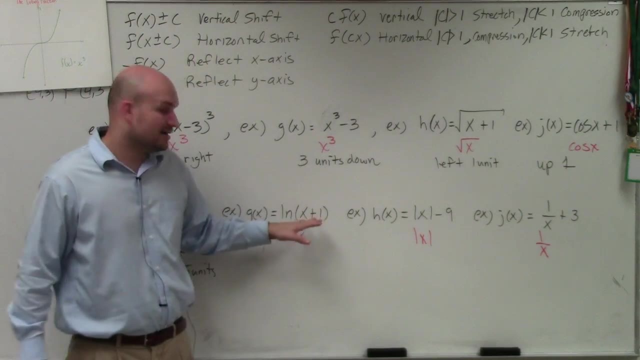 So, yes, it is inside, And since it's a minus, that means it's going to go to the right 5 units. That's why we're doing all this practice. Here I'm adding a 1.. You can see that it's going inside the function.